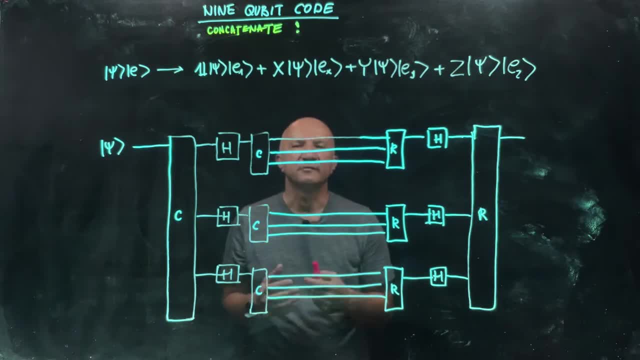 because if a bit flip error happens to one of the three physical qubits, you can recover from it. And you know the same story if someone comes to you and says: well, you know, protect against z-errors, but then you have to use slightly different encoding. So the question: 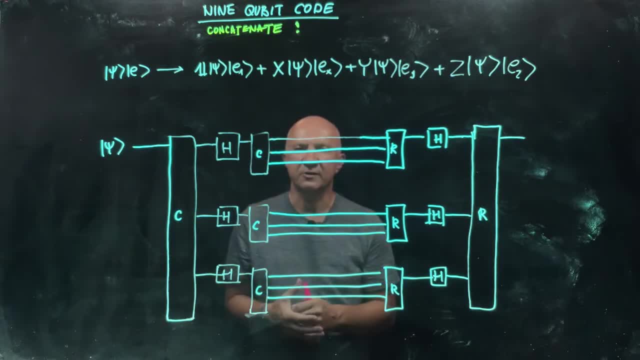 now is. someone comes to you and says, well, you know, protect against z-errors. but then you have and says, well, here is my precious qubit. Can you protect this qubit A little bit at least? Now you have to protect this qubit both against x errors. 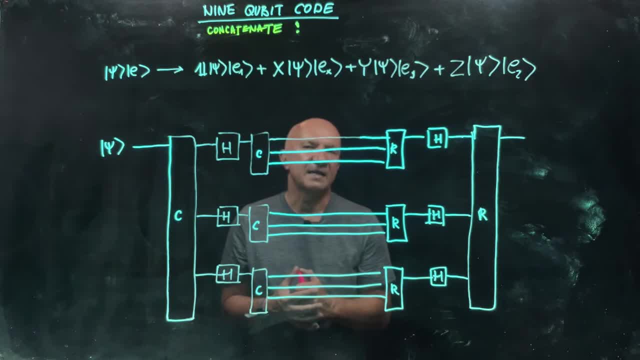 z errors. In fact, once you can protect against z and x errors, so phase flip errors and the bit flip errors, you can protect against any error whatsoever. And the reason for that is- you may recall from one of our previous lectures that if you have a single qubit in state, 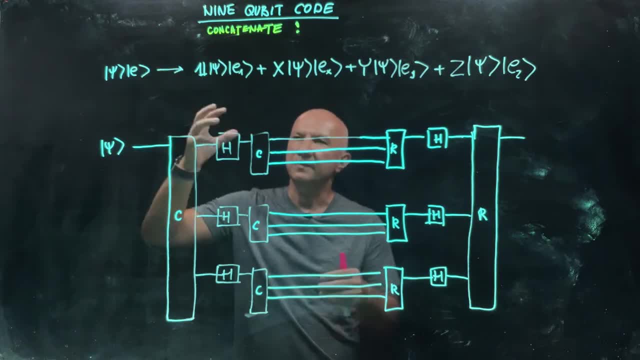 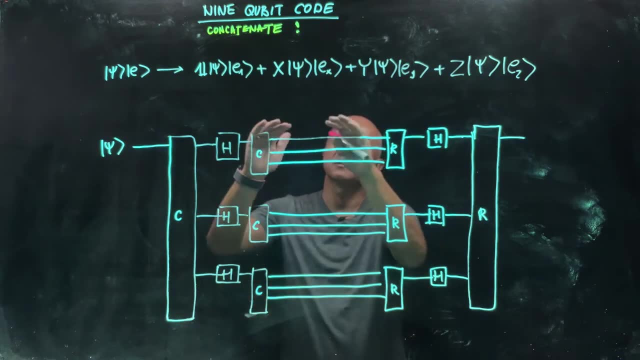 psi and the environment. in some state e interacting. the resulting state is an entangled state of your qubit and the environment. But the good thing is that this entangled state can be written in a way that admits a very simple physical interpretation. So you can look at the four terms in the superposition. 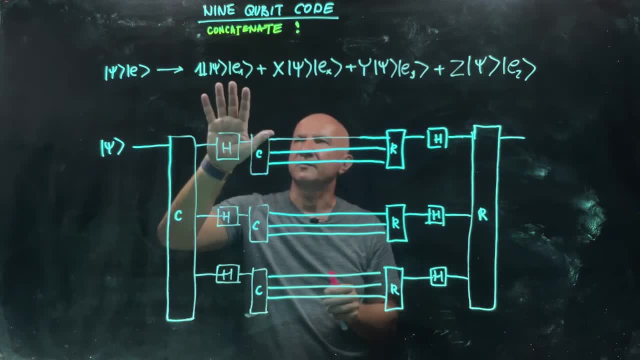 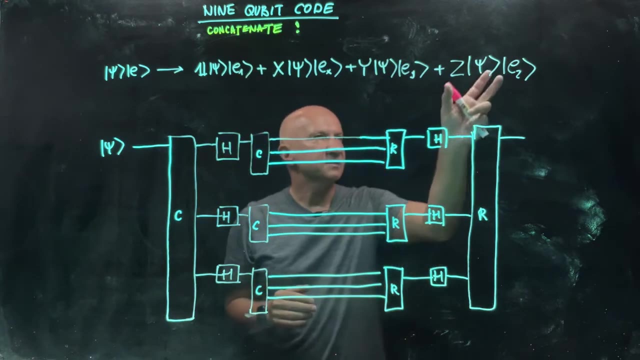 that I have here And you can see that the first term represents a situation where nothing happened to the qubit, so hence the operator, the identity. The second term represents the bit flip error, hence the x operator acting on psi. The last term represents the phase flip error, hence the. 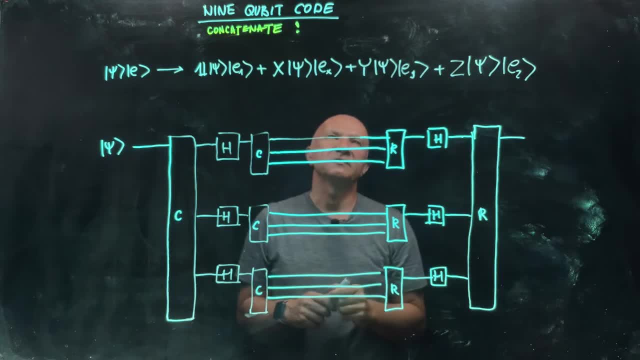 operator z acting on psi- And this term here represents both phase flip error and bit flip error, simply because operator y can be written as i x times z. So once we can correct Within the one system, once we can design a code that can 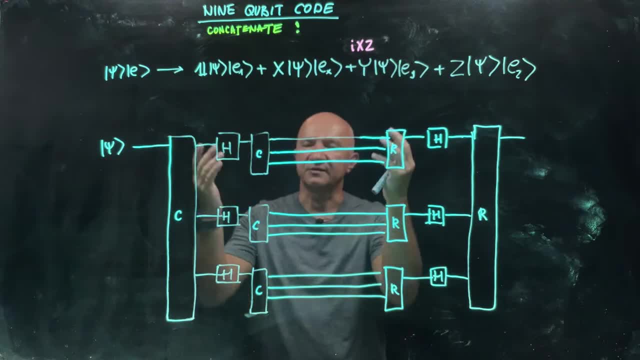 handle both bit flip errors and phase flip errors. we are essentially done. So how shall we do that? The idea is to use concatenation, to use two layers of encoding. So first encode your qubit to protect against the phase flip errors. 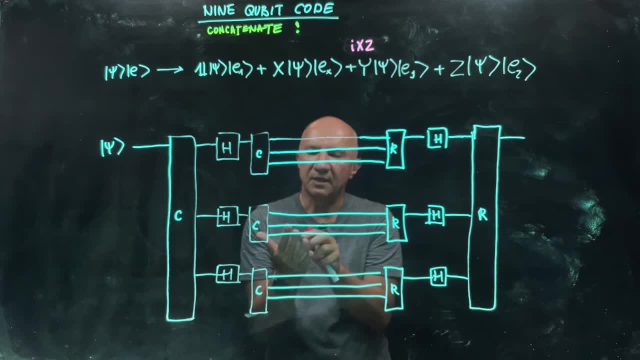 And then you have three physical qubits in the code, Take each of them and encode again, But to protect against bit flip errors. So here is the circuit And you can look at the circuit and you can see the pattern right. 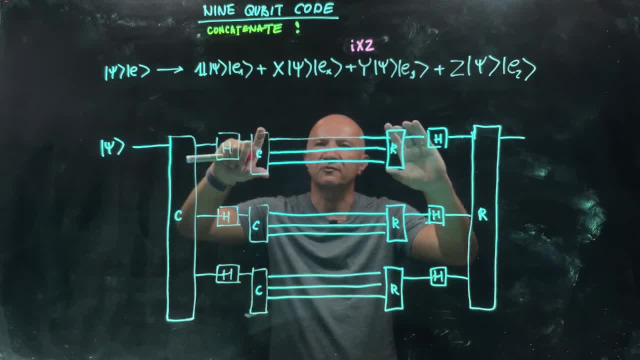 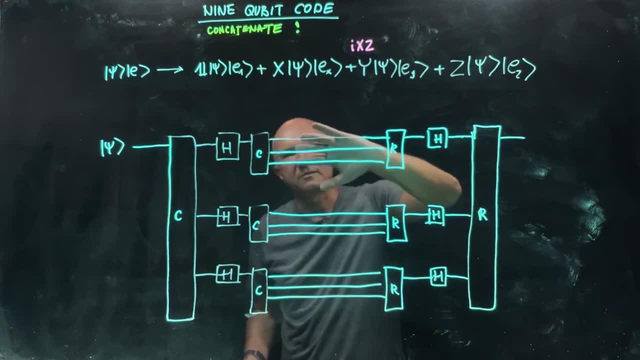 Here you have a three qubit repetition code correcting for the bit flip error, And the same here and the same here. So now, if you were to imagine those three qubits, think about the three qubits here as one logical qubit, and the 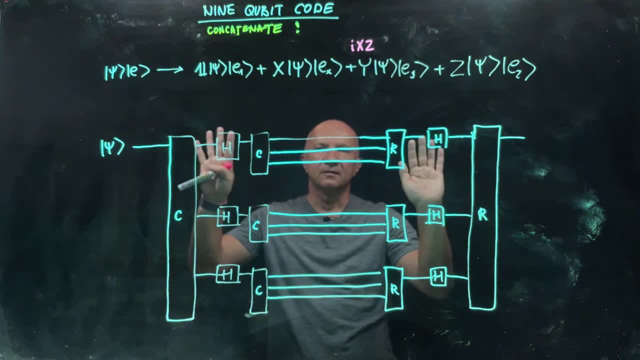 same here and the same here. So then you can just stand back and look at this pattern And you can see that in this case you would have a code, a three qubit repetition code correcting for the phase flip error. So for example, say, a bit flip error happens somewhere. 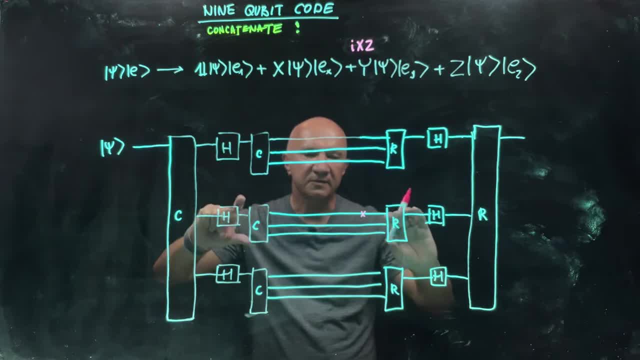 So say here No problem, right? So this code here, the three qubit repetition code that handles bit flip errors, will handle this error, The same if a bit flip happens on any other qubit. So there The inner layer will handle the bit flip errors. 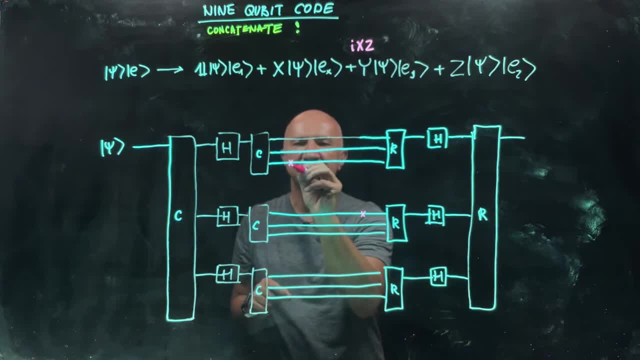 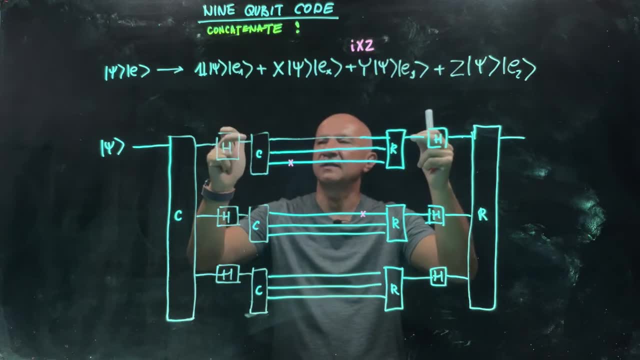 How about the phase flip error? So suppose you have a phase flip somewhere here. So clearly the inner layer will not handle the phase flip, but it will be delegated one level up. So if you then start thinking about this as one qubit one, 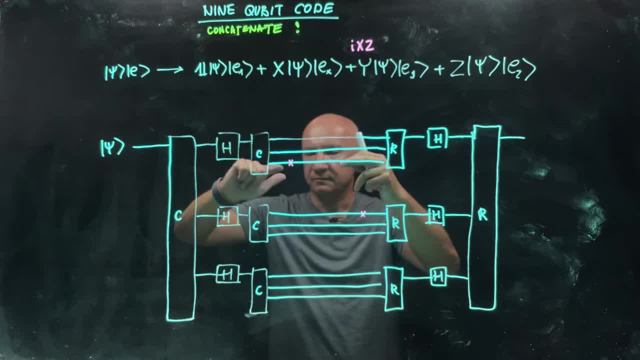 logical qubit, then this one logical qubit will have a phase flip error. So then the outer layer, The outer code, will handle the phase flip error. So, as you can see, by concatenating we have two layers of encoding here. 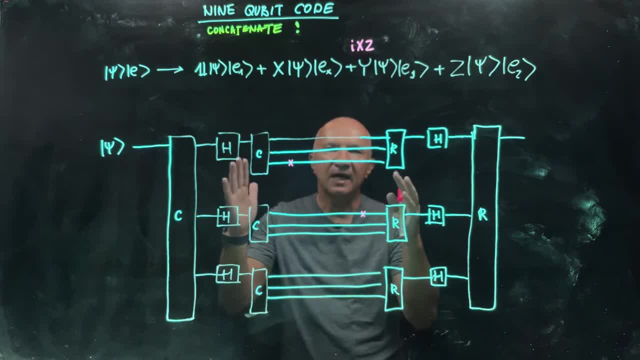 The inner layer that handles the bit flips and the outer layer that handles the phase flips, And that works beautifully. In fact, this code is much more clever than just correcting for a single bit flip error or a single phase flip error, So you may notice, for example, that the code is much more. 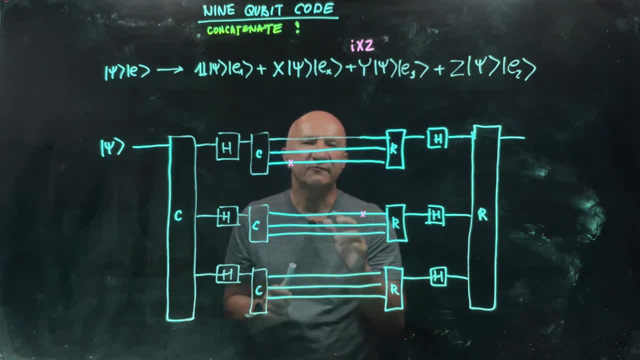 clever than just correcting for a single bit flip error or a single phase flip error. So suppose you have three errors, not just one error but three errors in the system. So you have a bit flip here, bit flip here and say bit. 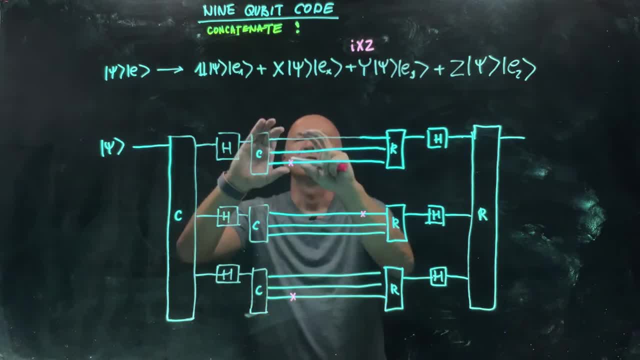 flip here. So all of them would be corrected right, Because this bit flip error appeared in this triplet that is associated with the bit flip correcting code. And the same here and the same here. So as long as the bit flip errors are spread over so that 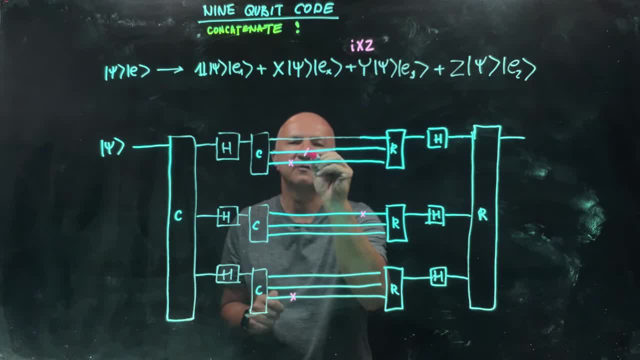 you don't have a situation, for example, where you have two bit flip errors within one unit, one triplet here. in this case you will not be able to correct such two bit flip errors. So you can look at this code and think a little bit. which? 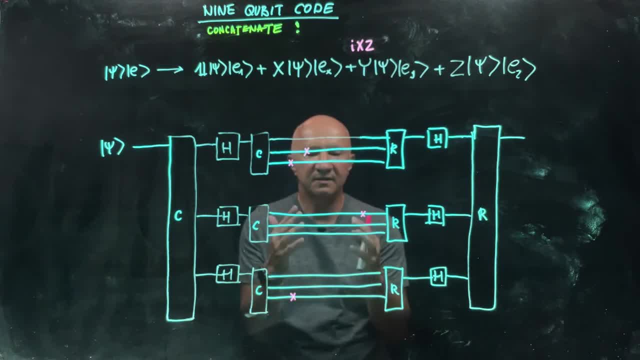 kind of errors will be corrected and which will not be corrected, But you can see that at least it can handle up to one general error. So this is one of the first codes that was proposed And of course, over time people came up with a number. 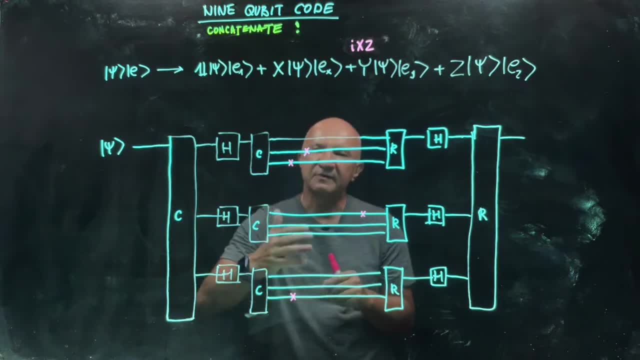 of interesting codes. So in fact you don't have to have nine qubits to encode one physical qubit and protect it against any error. So you can design a seven qubit code. You can design even a five qubit code. Actually, the five is the smallest number of physical 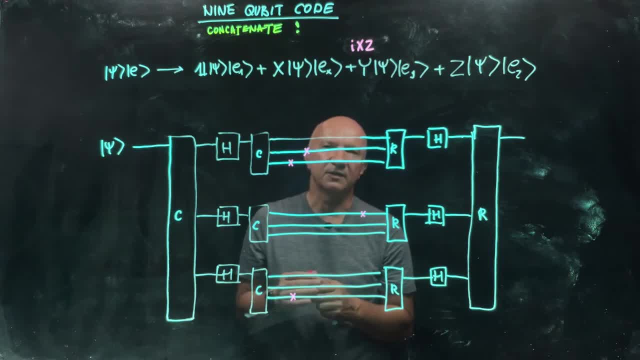 qubits that are required to protect your single qubit against any error, And we will talk about more general encoding. We may consider situations where, for example, you take not just one qubit and encode it into, say, nine qubits. 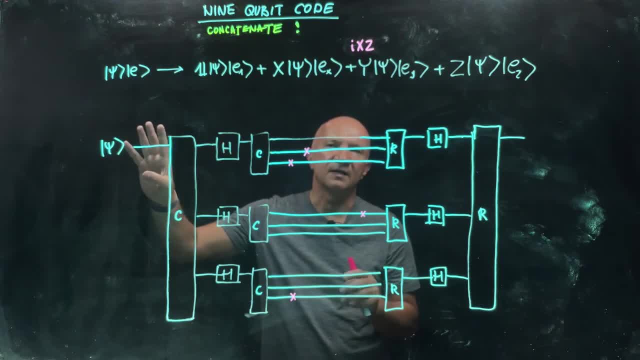 In general you can take n physical qubits and encode them into k physical qubits. So therefore you have n logical qubits represented by some number k of physical qubits. So one can study quantum error correcting codes of that time. Usually we take inspiration from classical error. 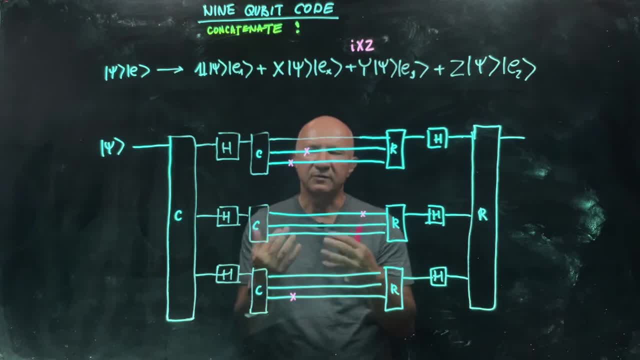 correcting codes and build quantum codes around them. We're not going to go into details. The whole field is actually thriving now because it is really important to design efficient quantum error correcting codes. But I think for the purpose of this lecture, I want you to